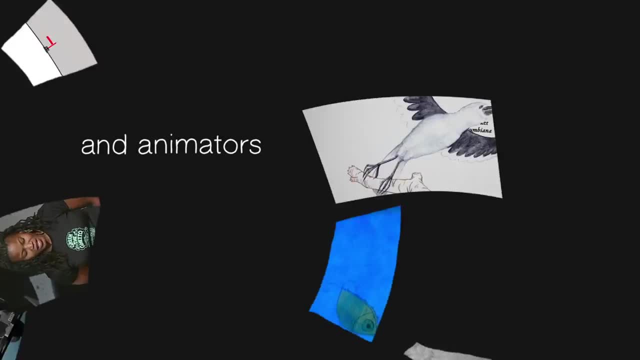 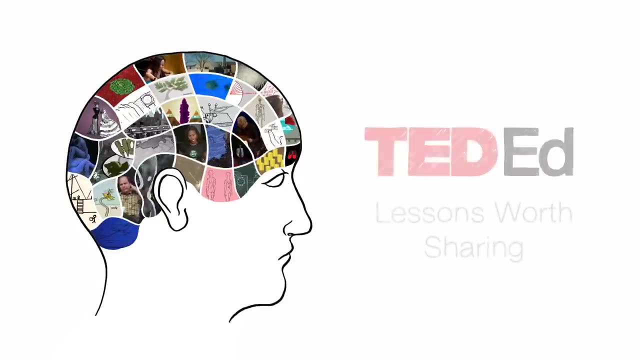 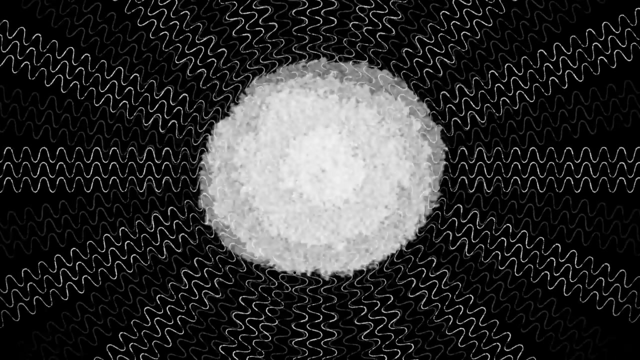 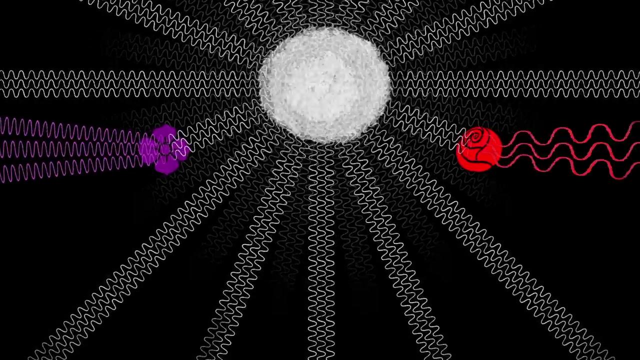 You might have heard that light is a kind of wave and that the colour of an object is related to the frequency of light waves it reflects. High frequency light waves look violet, low frequency light waves look red and, in between frequencies, look yellow, green. 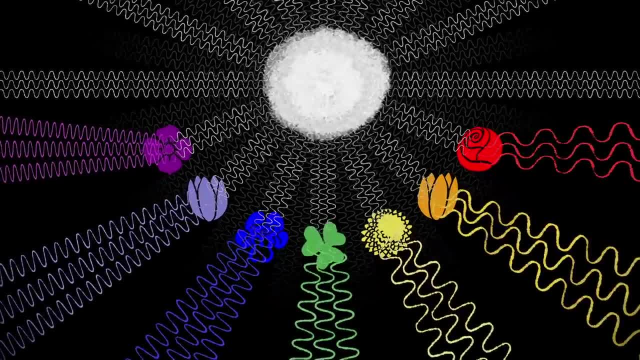 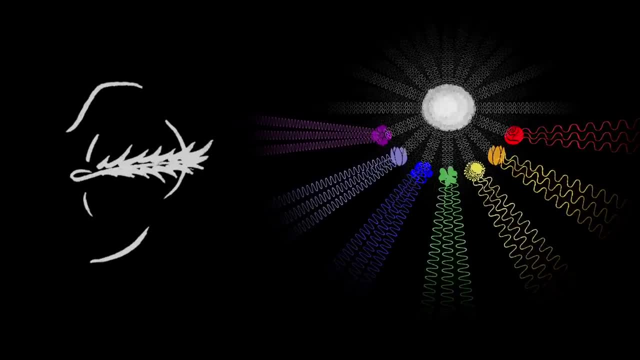 orange and so on. You might call this idea physical colour, because it says that colour is a physical property of light itself. It's not dependent on human perception. And while this isn't wrong, it isn't quite the whole story either. For instance, you might have 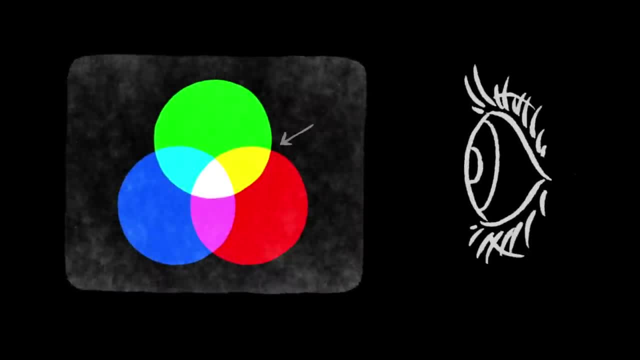 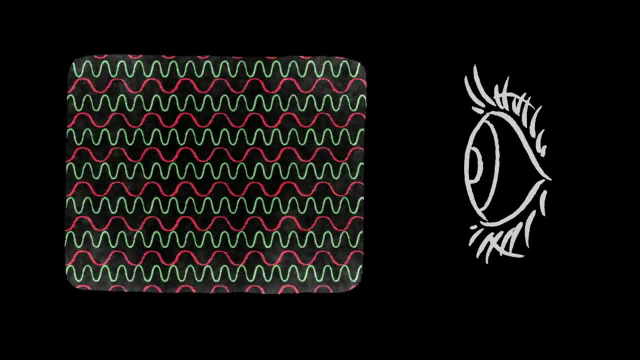 seen this picture before. As you can see, the region where the red and green lights overlap is yellow. When you think about it, this is pretty weird, Because light is a wave. two different frequencies shouldn't interact with each other at all. They should just co-exist. 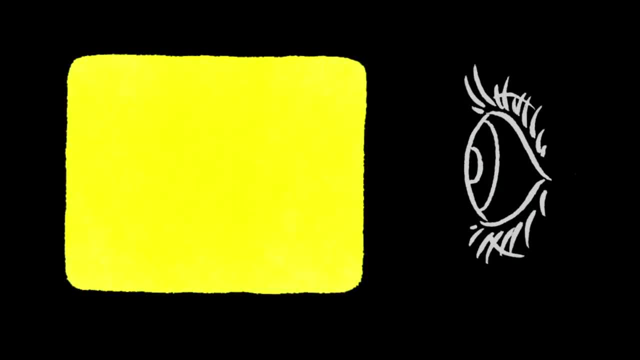 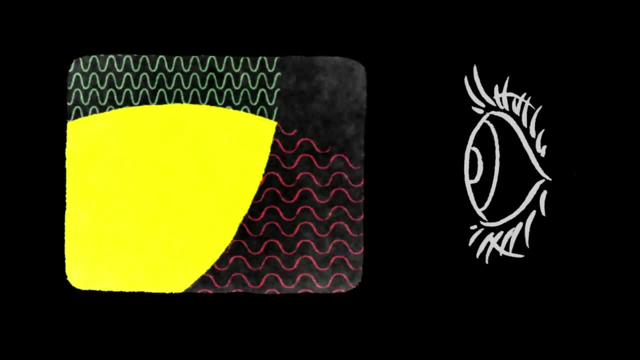 like singers singing in harmony. So in this yellow looking region, two different kinds of light waves are present, One with a red frequency and one with a green frequency. There's no yellow light present at all. So how come this region where the red and green 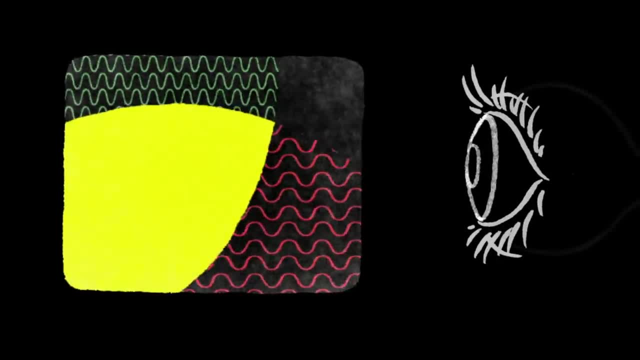 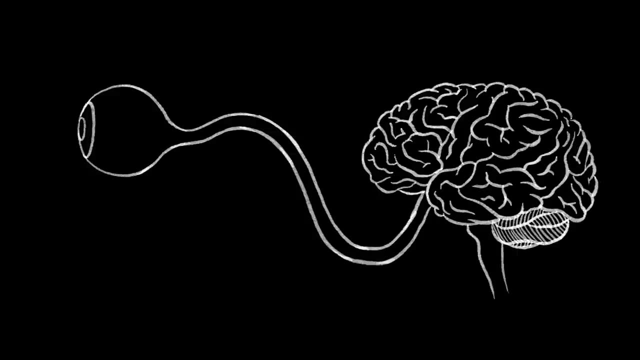 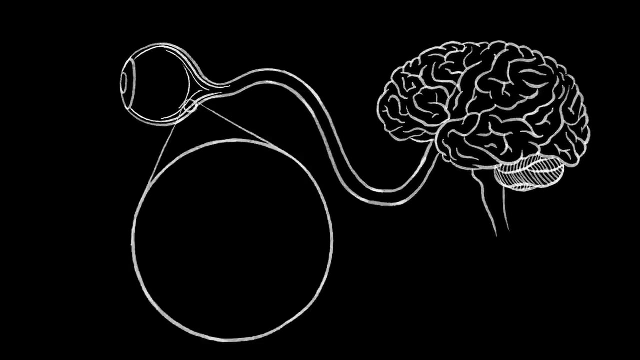 lights mix looks yellow to us. To understand this, you have to understand a little bit about biology, In particular about how humans see colour. Light perception happens in a paper-thin layer of cells called the retina that covers the back of your eyeball. In the retina there are two different types of light-detecting. 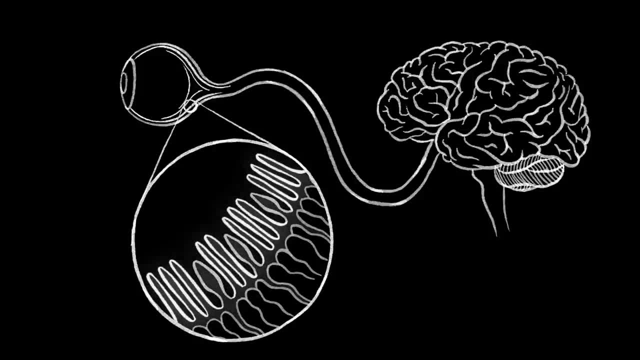 cells, Rods and cones. The rods are used for seeing in low light conditions, and there's only one kind of those. The cones, however, are a different story. There are three kinds of cone cells that roughly correspond to the colours red, green and blue. When you see. 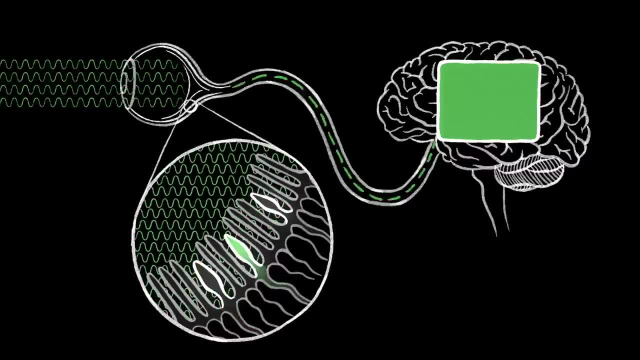 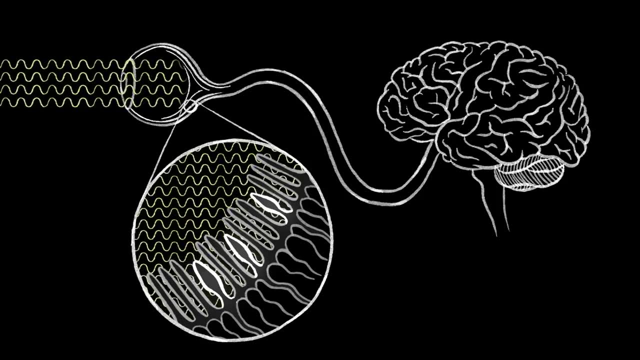 a colour. each cone sends its own distinct signal to your brain. We're going to look brain. For example, suppose that yellow light, that is real yellow light with a yellow frequency, is shining on your eye. You don't have a cone specifically for. 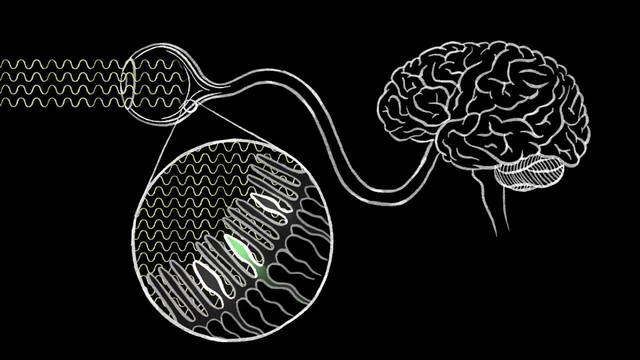 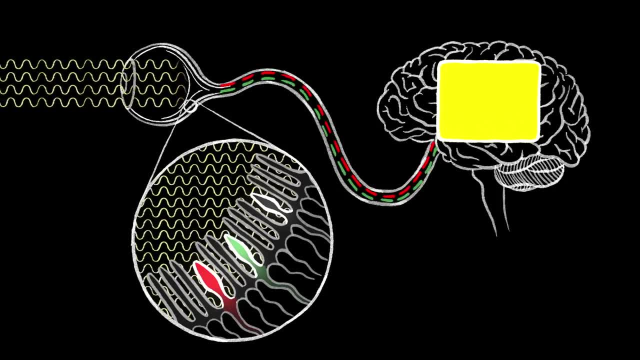 detecting yellow, but yellow is kind of close to green and also kind of close to red. so both the red and green cones get activated and each sends a signal to your brain saying so. Of course there's another way to activate the red cones.